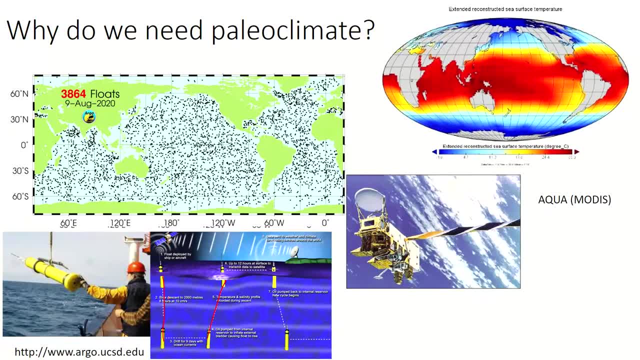 of information about the depth profiles of physical properties, temperatures, salinity, Because they drift around. they also tell us about ocean currents. I already mentioned we get a huge amount of information from satellites, So the present ocean is actually remarkably well instrumented. We know a huge amount of what's going on at 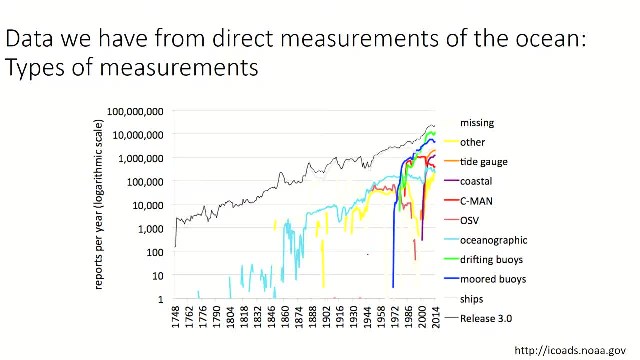 the moment, But if we look kind of back in time. so this is a graph of showing us how much data is collected in the ocean or from the ocean, from direct measurements of the observations. So these are things where an object, some kind of sensor, is going into. 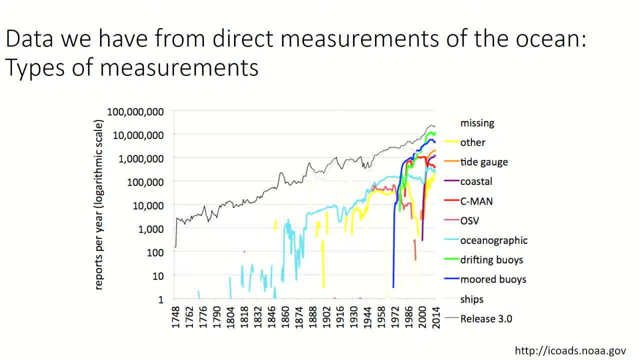 the ocean and that can be a thermometer or a conductivity sensor, or someone is scooping up a bit of the ocean and then measuring that And you can see how that's changed through the years. I guess this compilation only goes to 2014.. But you can see, in the 1750s we 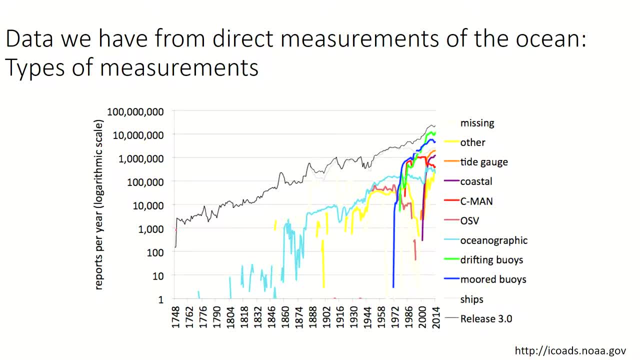 were only maybe getting a thousand observations of the ocean a year, And these largely came from ships recording the temperature of the water, maybe the wind direction or pressure, as they kind of sailed around the ocean. And as the density of shipping has gone up, the number of observations has steadily increased through time, I should 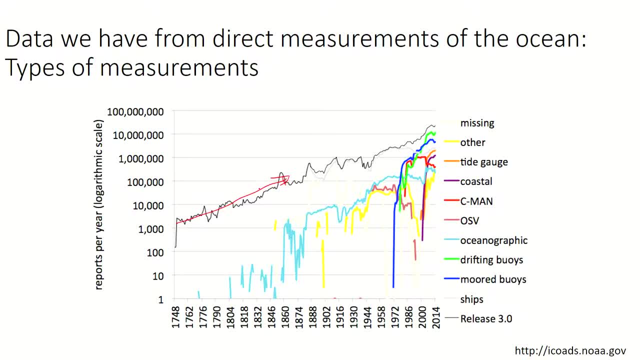 point out that this is a logarithmic axis, So this straight line on this graph would be an exponential increase in the density of observations. So I just point out that all the colored lines on here are all the different types of observation or the types of measuring platform. The black line on top is the total and the 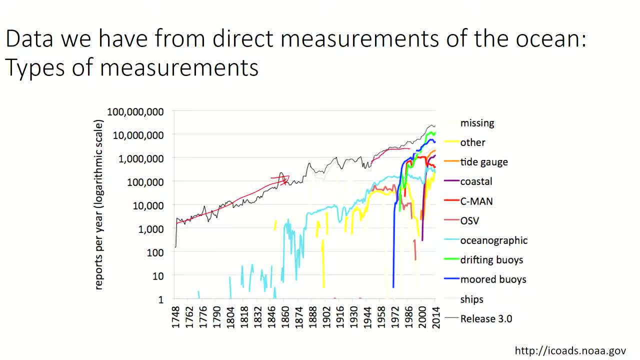 gray line which is here. that's kind of measurement for ships And you can see. what's quite interesting is that through the whole history of oceanographic measurements, from the 1750s up until, I guess, the 1990s- 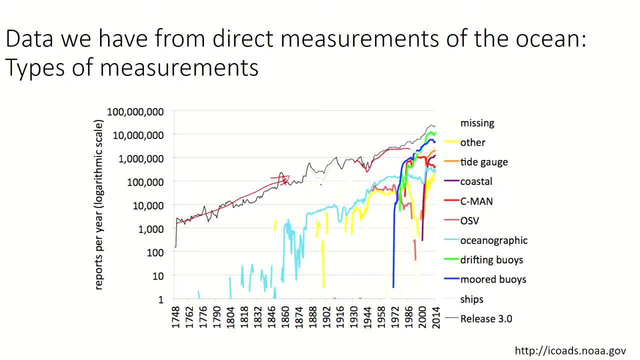 The vast majority of measurements were measurements of ships, people going out and making measurements, But you can see here since I guess the mid-90s at this point here we can see that these two other sources have overtaken the ships as the most abundant data source And that 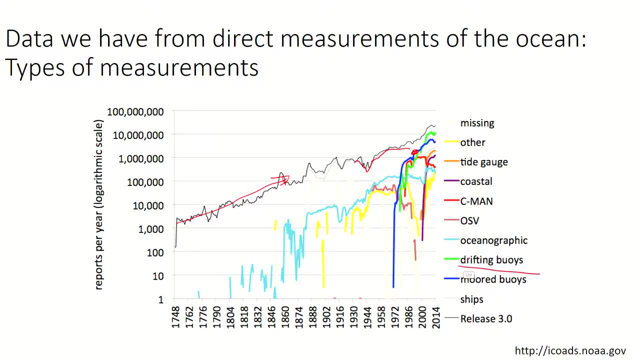 are these drifting buoys- that's a straight line- these drifting buoys here, And that's the most abundant data source, And that's the most abundant data source, And that's the most abundant data source. So these are those Argo floats And also buoys which are kind of like fixed in position. 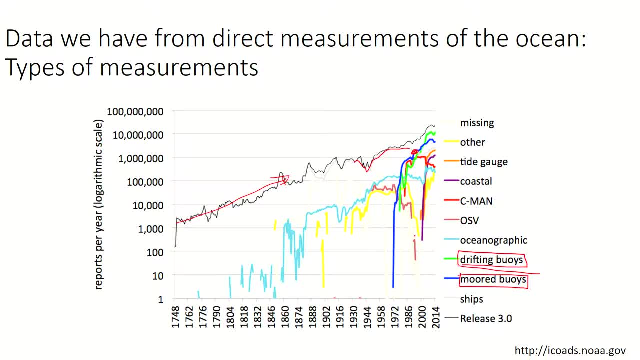 in the ocean, constantly kind of measuring at any one locality. So ships going out on ships is still important, but the vast amount of data we're getting from autonomous platforms, But that high density of data you can see only really goes back a few decades or so. 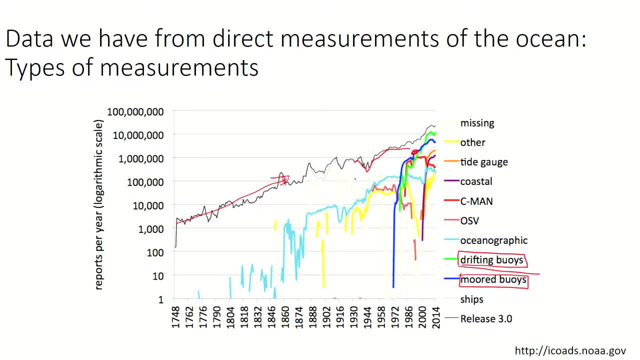 So what we can see from this is that, although the amount of measurements we're getting from the ocean is quite large- tens of millions of measurements per year- those data don't go back very far in time in that kind of density, As we go back 100 years or so to the beginning. 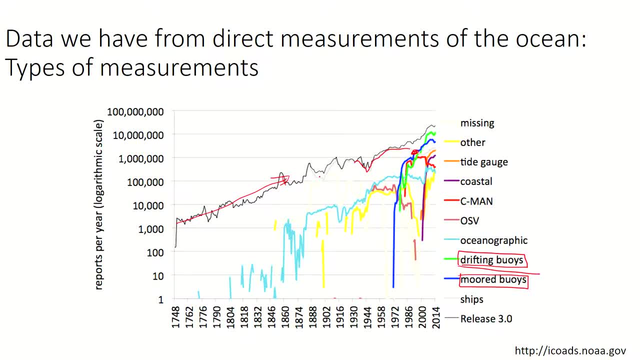 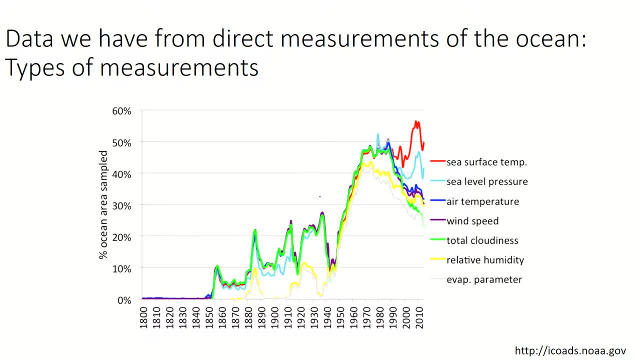 of the 20th century, we're down to maybe hundreds of thousands of measurements per year rather than millions. We can also see that the range of measurements that have been made so, rather than looking at the platforms that they were measured from So predominantly, we can see here that actually because the data density is lower as we go. 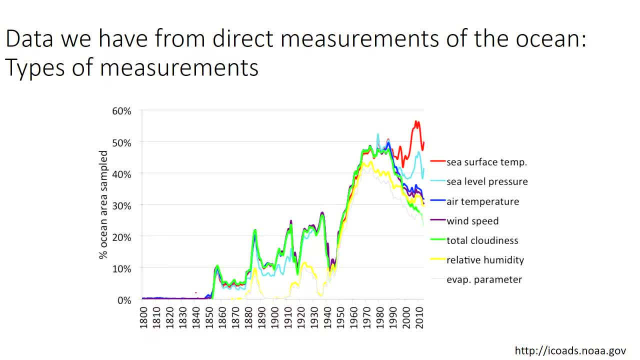 back in time. if we look at the amount of ocean that's actually been sampled back in kind of the- I guess, the 19th century here I guess we're looking at. less than 1% of the ocean has been measured. 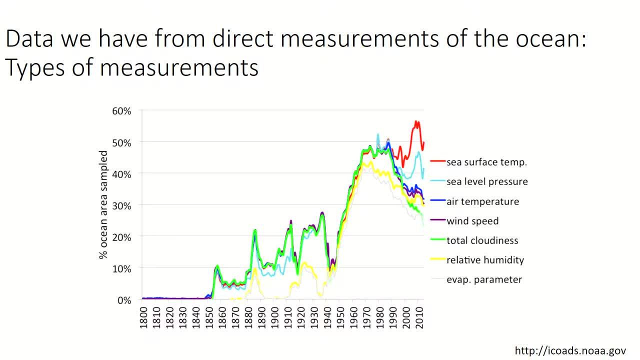 So we know very little about the ocean. that far back in time It's looking quite good- over 50% of the ocean measured, I guess now we know about that, but we're really limited to some, I guess, easy to measure. 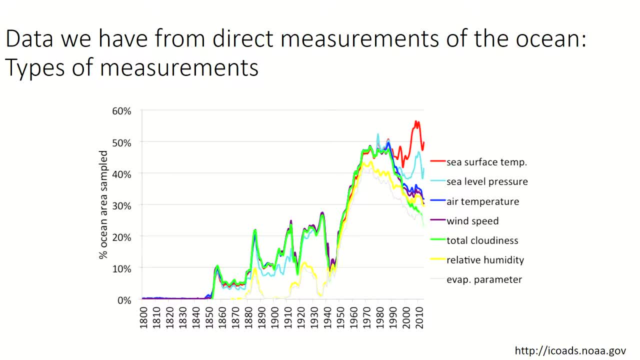 parameters, things like sea surface temperature, pressure, air temperature. So these are really measurements that were made for the purposes of meteorology, so to understand kind of the weather rather than to understand the ocean. So we're quite limited with the range of measurements that have been measured back in time. 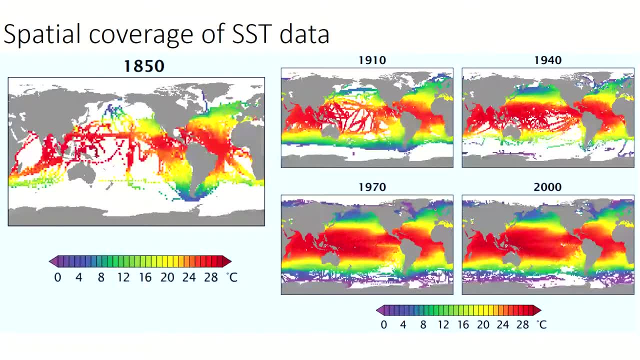 And just to kind of like hammer home that, that spatial distribution of measurements. so we're really limited to where I guess people were going in ships that have thermometers on them. So you can see that in, I guess in the 2000s, even in the 1970s, the ocean is quite well. 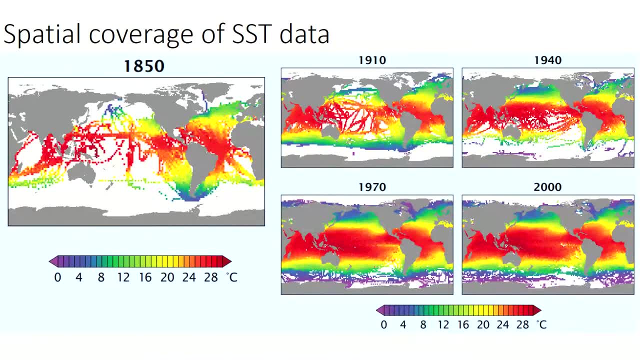 covered, in terms of its measurements of sea surface temperature Back into the 19th century, huge parts of the Pacific Ocean. here I mean not really measured that well. The Southern Ocean, not really measured at all, Not really that we're going to be able to fill in that gap in the Southern Ocean with. 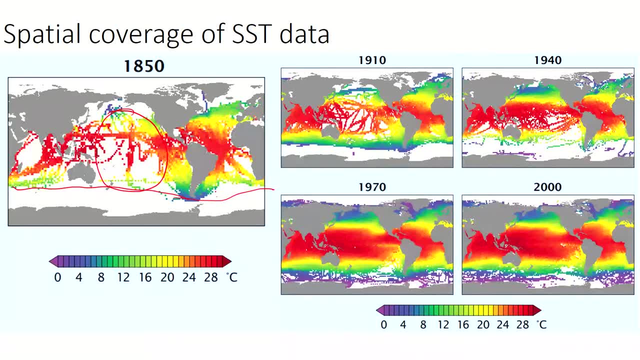 corals. There's not that many sea surface-dwelling corals that live in the Southern Ocean, But there are large parts of the ocean which we basically don't know about or don't know how their oceanographic conditions were. oceanographic conditions were back in time even only. 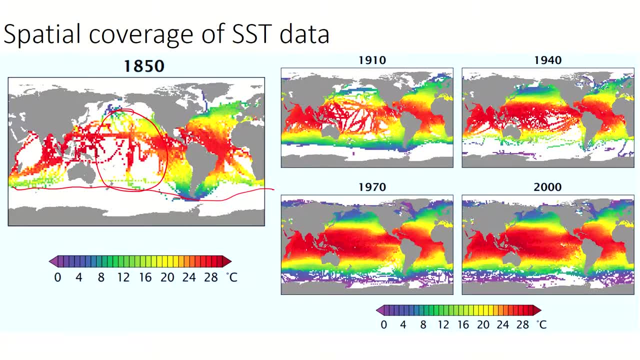 100 or so years. So again we're really limited with the measurements that were made for the purposes of meteorology. so to understand kind of the weather, rather than to understand the weather And just to kind of like hammer home that I guess in the 19th century huge parts of 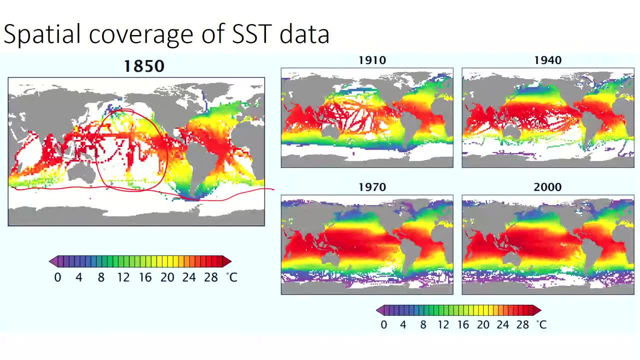 the Pacific Ocean- here I mean, not really measured that well. The Southern Ocean, not really measured at all. There's not that many sea surface-dwelling corals. There's not that many sea surface-dwelling corals And just to kind of like hammer home that I guess in the 19th century huge parts of 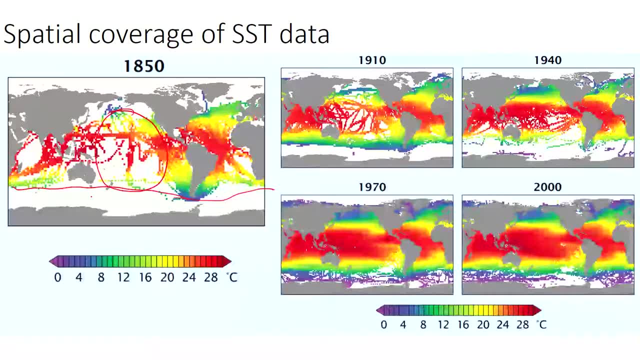 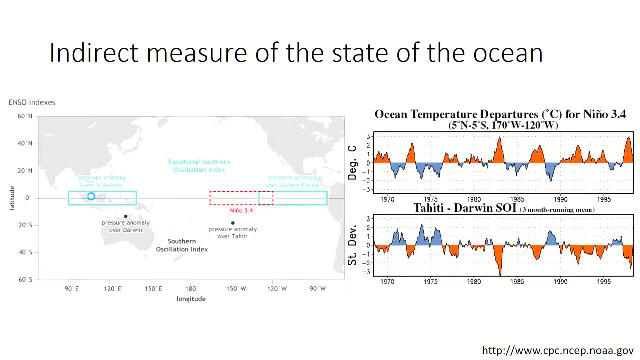 the ocean which we basically don't know about or don't know how their oceanographic conditions were. oceanographic conditions were back in time, even only 100 or so years. So another potential way that we can maybe get round this problem is by using some of 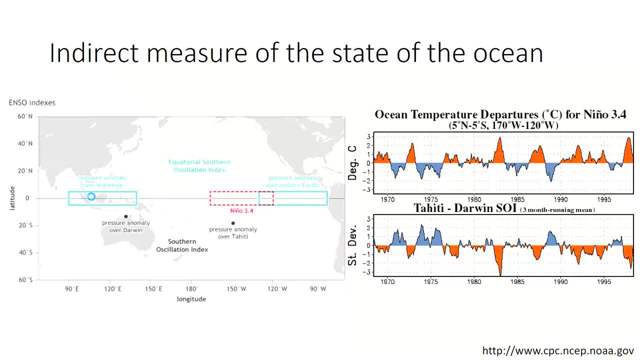 this meteorological data that's actually that's been collected for a reasonably long time, in terms of, I guess, 70 or 80 years, uh, the industrialization of the planet, um, but maybe not geologically a long time ago, when people from people mostly from, i guess, uh, asia and, um, western europe, started to make meteorological 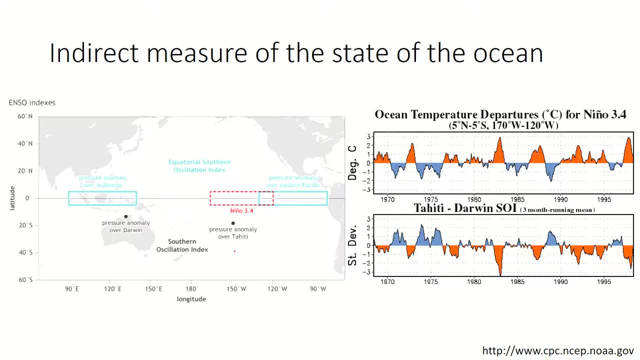 measurements. so, looking at maybe going back hundreds of years, uh, we can use measurements of particularly things like sea, uh, sorry, atmospheric temperature and pressure, because those parameters, uh, in some situations can quite closely correlate with the oceanographic conditions. so this is an example which i guess may be familiar from. uh, the brief introduction to the el. 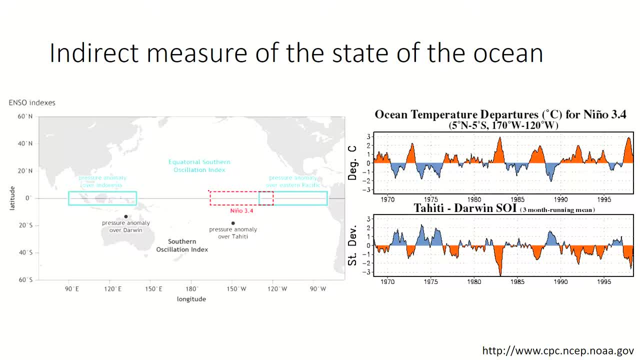 nino southern oscillation: um, so, uh, if we wanted to know what the temperature of the ocean in this box here was back in time- we don't really have that many uh, measurements going back hundreds of years- uh, of, um, of, um, oh yeah, anything going back there, because we weren't there measuring the temperature. 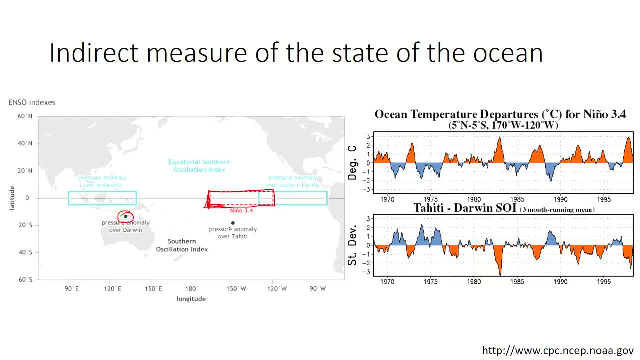 uh, but what we can do is, if we measure the sea level pressure in darwin and tahiti- uh, i mean, there have been meteorological stations, uh, these two locations for many, many years now- we can see that the the sea level pressure here, so that's pressure here, that quite closely. 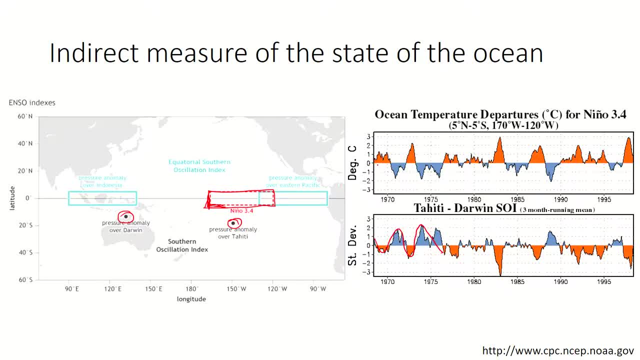 correlates with the ocean temperature in this, this box, so we can use, i guess, indirect, don't direct, i guess real measurements, but indirect measurements of the ocean to understand about how the ocean has changed in the past. but i guess this is, i guess, a step removed from actually. 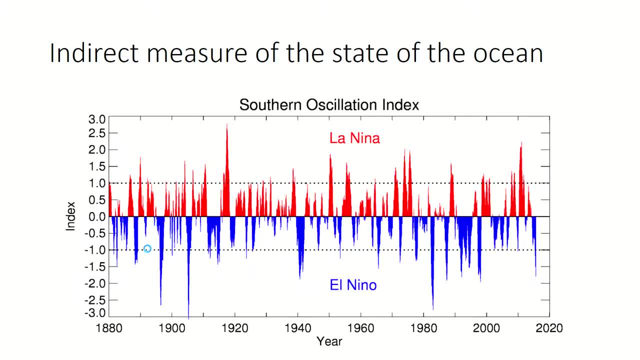 measuring um, yeah, so this is, yeah, example of exactly that. so we actually have a record of this pressure difference going back, i guess, almost 150 years now, giving us quite a long record of the, i guess, the the state of the um, of the ENSO, the El Nino Southern Oscillation System, which is quite neat. But we can't do this. 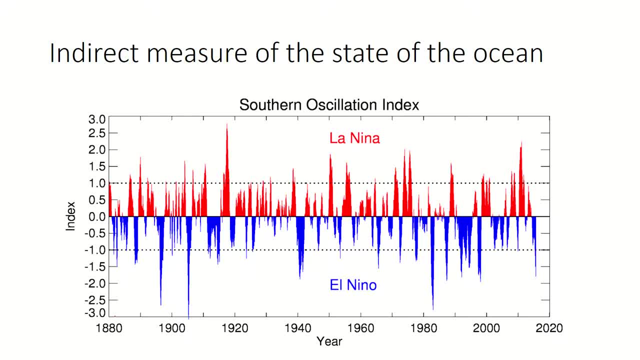 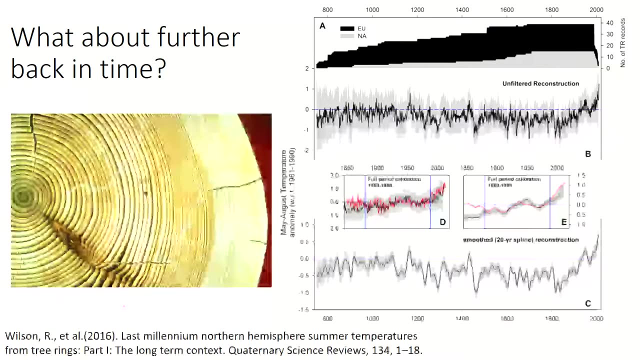 for all parts of the ocean, and we can't do this, I guess further back in time, from when, I guess, Europeans started to come to these places and build meteorological stations, amongst other things. So this is where we start to go into the paleoclimate proxy world. So this is an example. 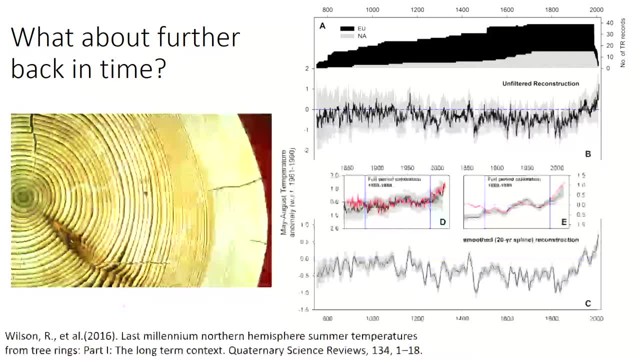 I guess from the terrestrial realm, where scientists have used tree rings. So tree rings are very useful because they're very easy to count, so we can work out exactly how old a particular ring in a tree was. so we can basically count back the rings and get the age, and then we 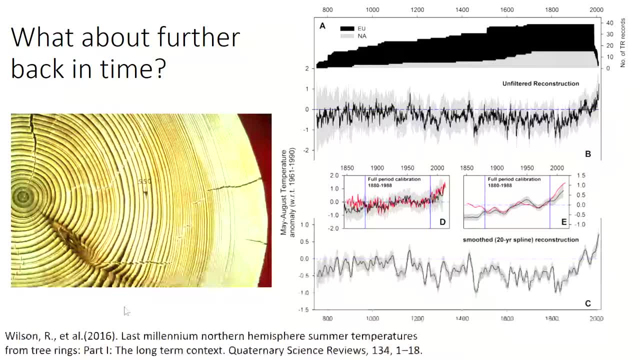 can use the thickness of the ring to tell us something about the climate in which that tree grew. So it's a particularly thick ring that might indicate they're warm or wet or very productive growing year, whereas it was a very thin ring that might indicate that colder, less. 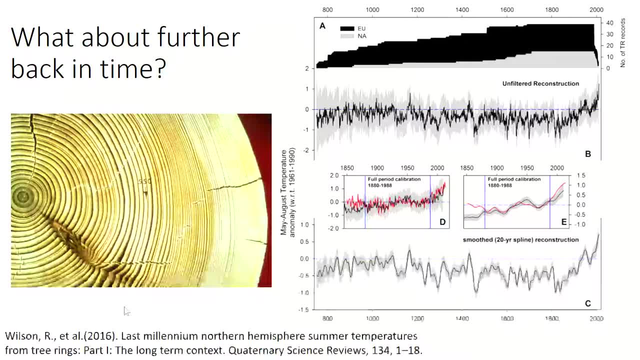 suited for tree growth, And we can build big compilations of these and we can use that to reconstruct the regional temperature where that tree grew, back in time. and this is effectively what's been done to work out the surface temperature of the planet back. I guess, almost I guess- this is a complex that only goes back 1200 years, but I think we've gone back. 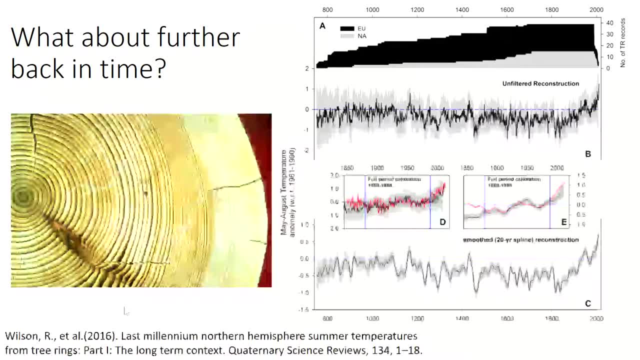 2000 years to illustrate how variable the climate has been over, I guess, the last thousand years and how anomalous the warming are present. So we can use, I guess, what we call proxy measurements, where we're measuring some kind of thing that occurs in some kind of medium. In this case we're measuring the thing is the. 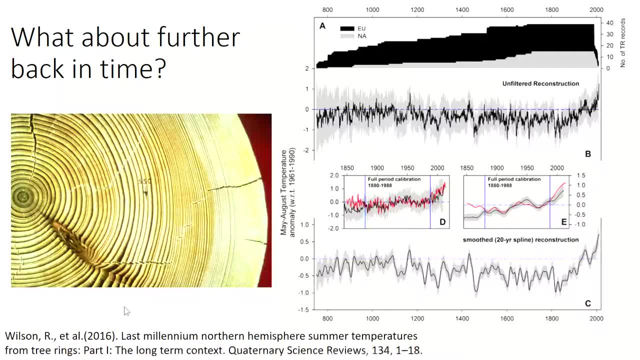 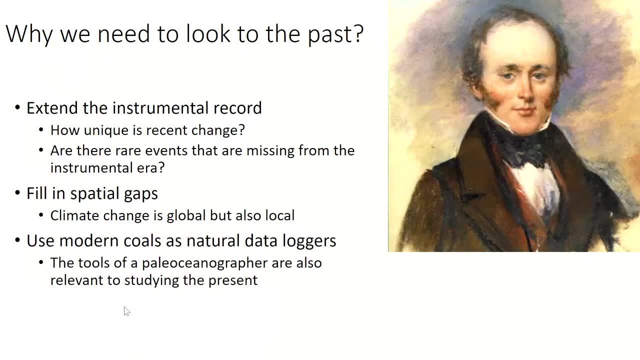 thickness of the rings in the tree, and that tree is the medium and that we're using as a proxy for the local environmental conditions. So we are going to look at a variety of different proxies throughout the rest of this section of videos. So we're looking into the past because we can. 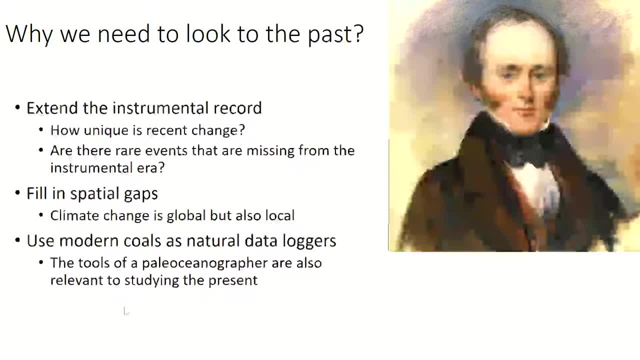 extend that instrumental record. we can look further back in time to get a longer time series which will allow us to really say whether a particular climate phenomenon is anomalous or not. it might allow us to see different kind of climate behaviors which we've not yet observed in the instrumental record. We can also use this where there 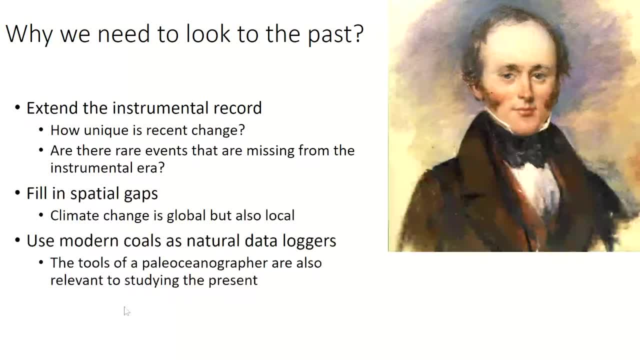 aren't any instrumental records because, for whatever reason, Europeans with weather stations didn't rock up and record all of the information. So we're basically using these proxies of past environmental conditions as data points. And the image I've got up here is this guy, Charles Lyle, who was, I guess, Edinburgh scientist and one of his- I guess his- key ideas. 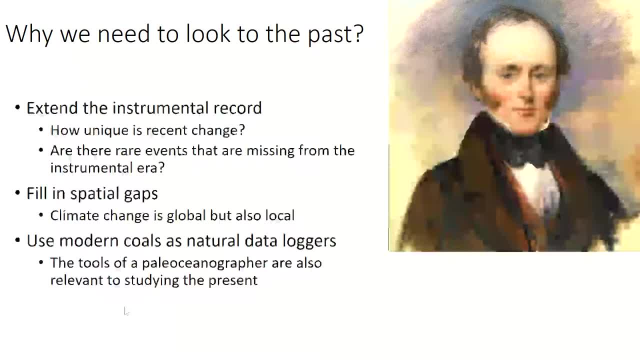 in the Scottish Enlightenment was that you could use the present environmental conditions to understand kind of like rocks and the past. But actually we can. we can use that the other way around and we can use the past of, I guess, rocks, corals are lots of them. 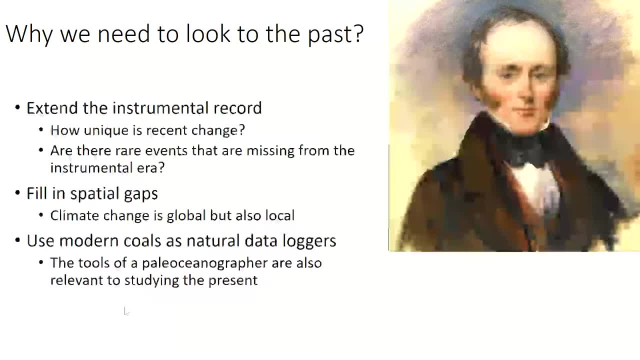 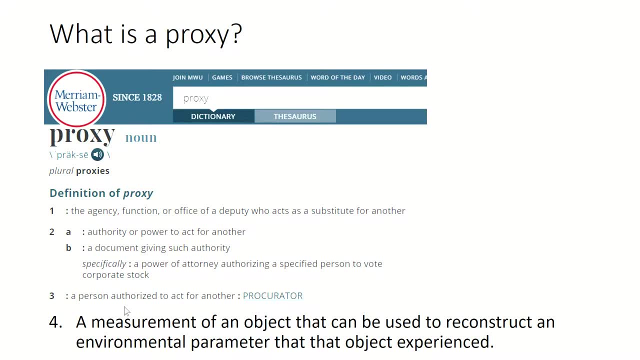 to learn about how the earth works. So yeah, so just to get some dictionary definition of proxy is so you might have heard the word used, as I guess, in a variety of different settings in terms of someone that acts on behalf of another person, in terms of, maybe, proxy voting. 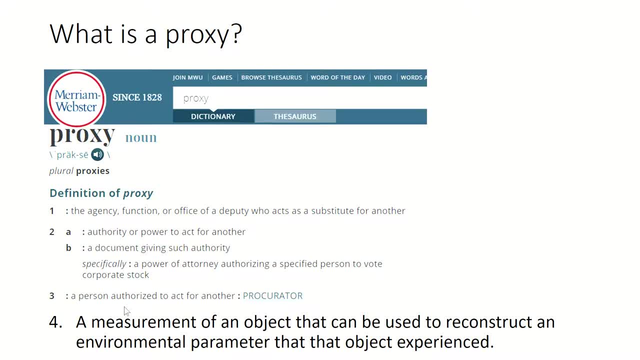 or maybe kind of a political proxy actor or something like that. But actually we're adding in this kind of additional term. so it's a measurement of a physical object that we can kind of extract from the geological record and something that we can measure in that to. 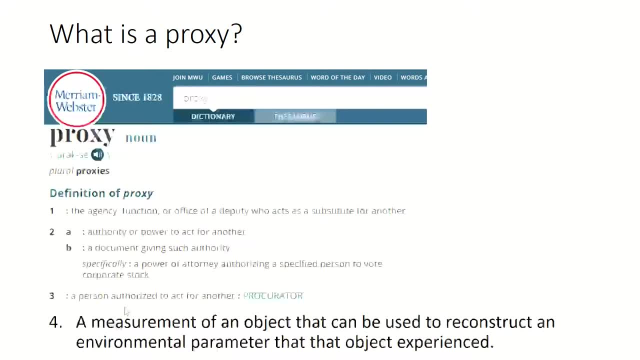 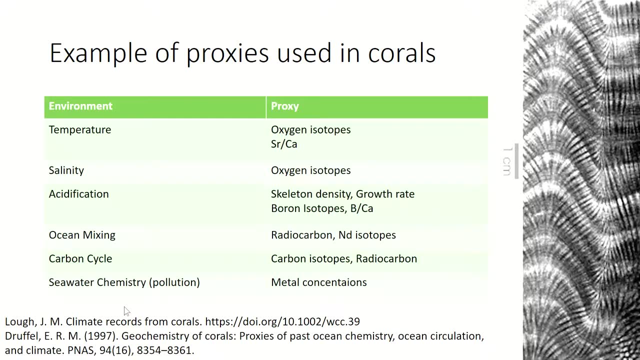 reconstruct an environmental parameter, and that could be temperature, salinity or a variety of other things. So just to give some examples- and we'll go through these kind of in separate videos into how these these work and some examples that are being used. So, for example, we could want to: 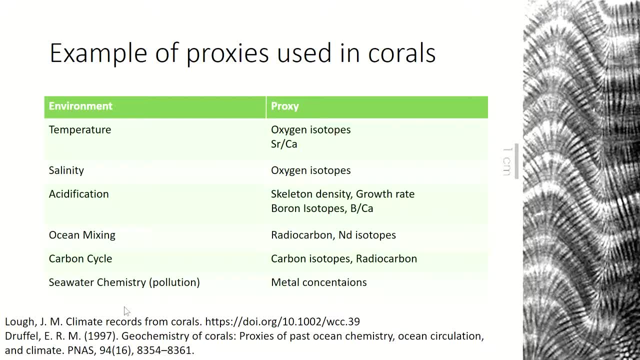 reconstruct a temperature in which a coral grew, and we might use its isotopic composition of oxygen preserved in its skeleton, or the proportion of strontium compared to calcium in the mineral structure. We might want to reconstruct how acidic the ocean was. There are a variety of different. 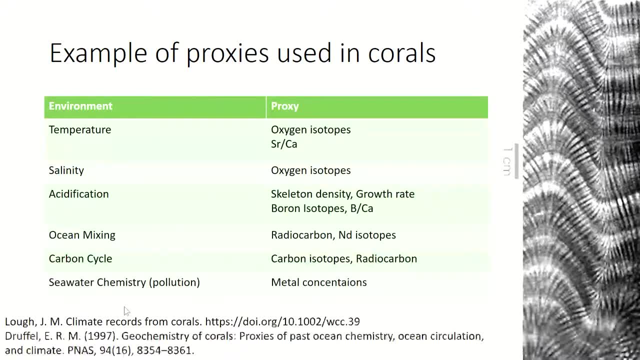 kind of physical properties of corals but also chemical and isotopic measurements that we can make in those. So we'll go over each of these kind of in turn. but basically the summary of this introduction is that using kind of paleoclimates, using proxy, 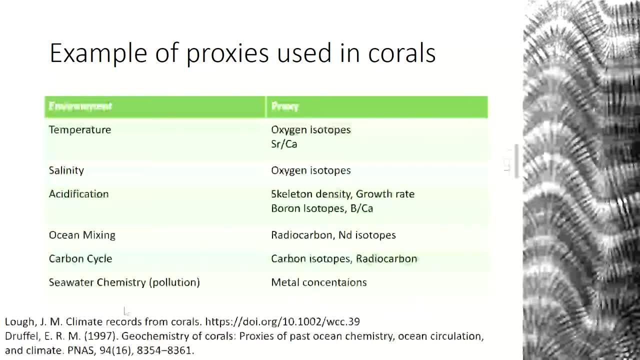 measurements of the past ocean conditions, if possible, is really useful because it allows us to extend our knowledge of the ocean back in time to times when we didn't have a wealth of data that we have from direct measurements, and it also allows us to go and sample spatially exactly where 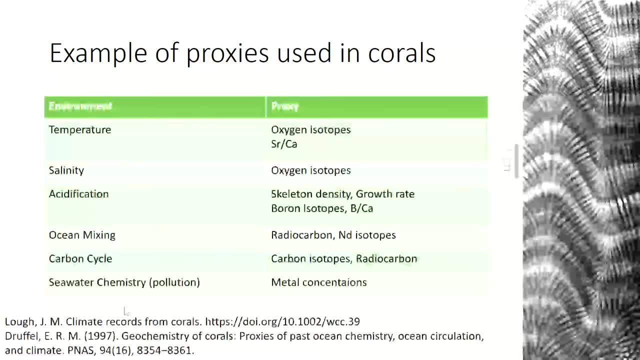 in the region we want, or to what we're interested in, without there having to be a weather station that has existed there for you know, many hundreds of years. Right, we'll stop there and the next kind of few videos. we'll go through each of these, these different systems, how they work, and some examples. 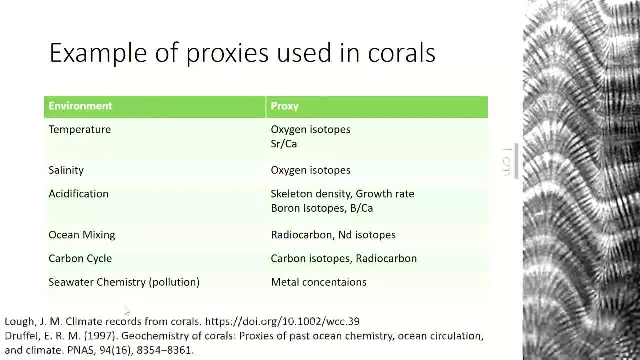 of, I guess them working. So that's us done for this video.